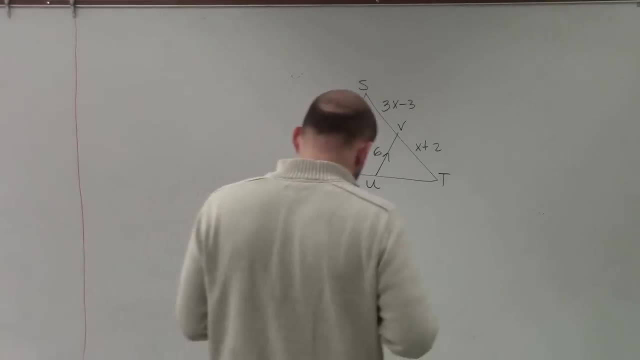 So what they're asking, ladies and gentlemen, in this problem is identify the similar triangles, then find each measure. So what we need to do again, when we're doing a problem like this, we're going to go ahead and do it. a problem like this. 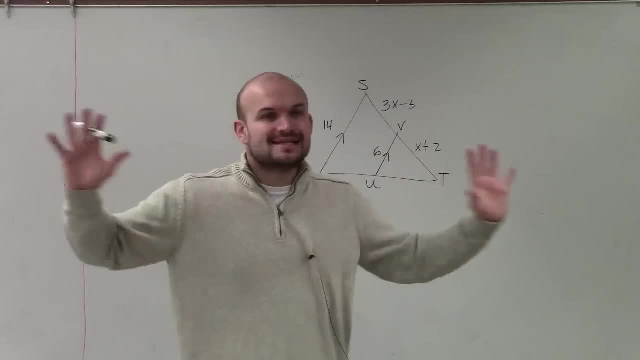 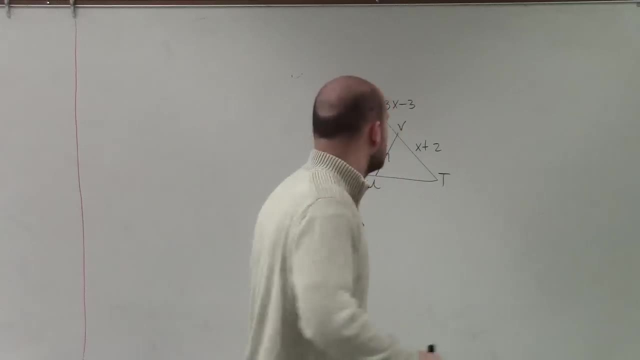 The main important thing that I told you guys is to take away the triangles right. Separate the triangles so you can see them, Carly, as their own identity, not trying to determine what is one triangle over the other. So I am going to draw them separately, all right, and then go ahead and label them SRT, all right. 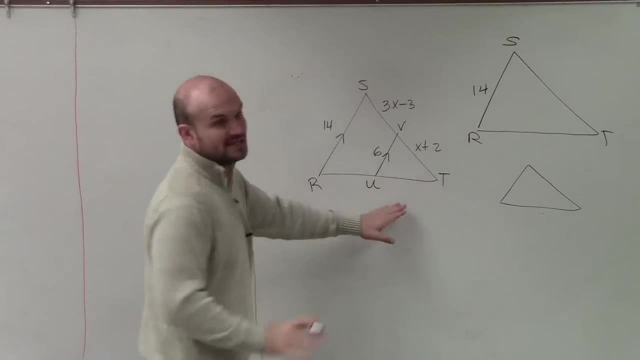 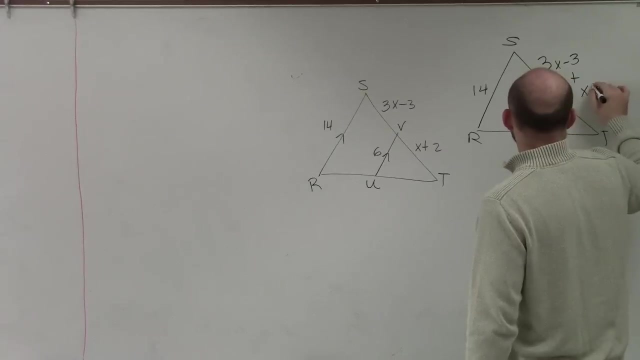 So this length is 14.. We don't know what this length is right, But we know that this length is going to be 3x minus 3 plus x plus 2.. Would you guys agree on that, Caleb, do you? 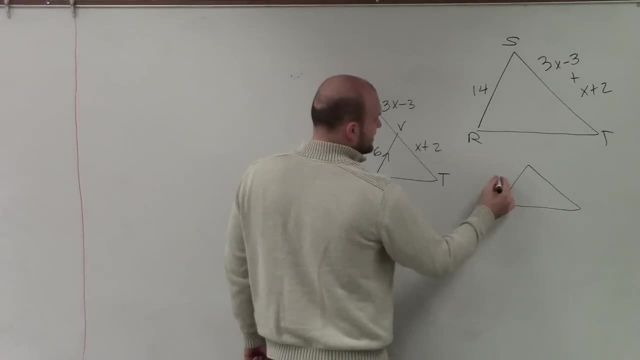 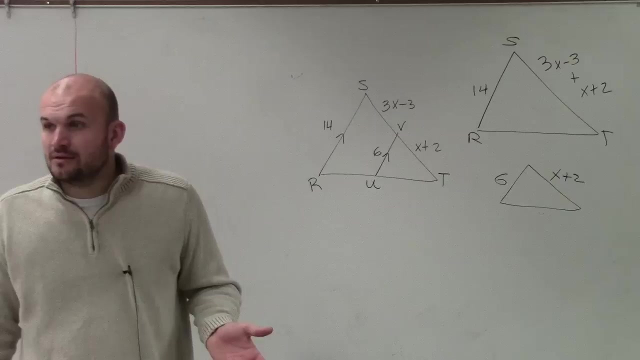 Agree on that. Okay, Over here you could say: this length is 6, and this one is x plus 2.. So what we're trying to do is they say they are similar, but how are we going to be able to? if they're similar, then that means their side lengths, right, are proportional. 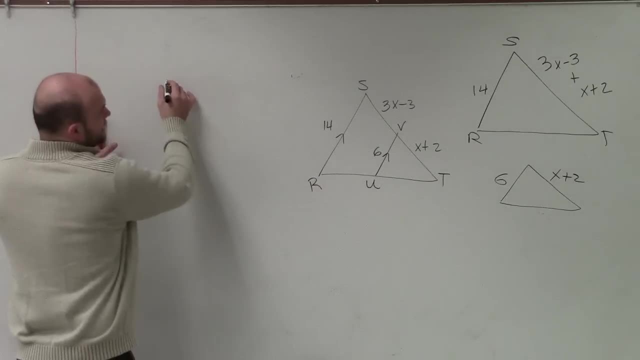 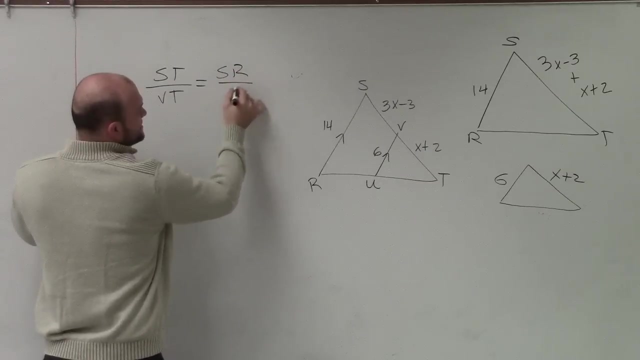 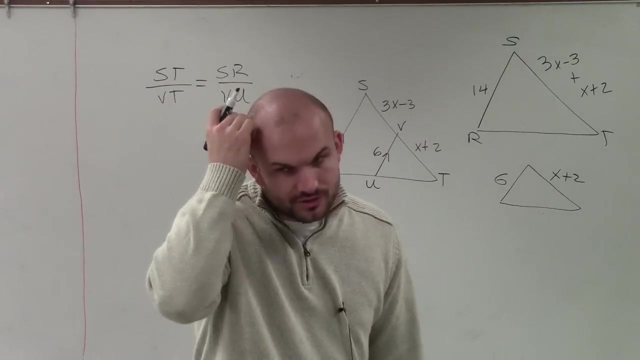 So what I can say, then is I can say: ST is to VT is equal to SR is to VU. All right, Their side lengths are going to be proportional to each other. So now what I need to do is just plug in their side lengths. 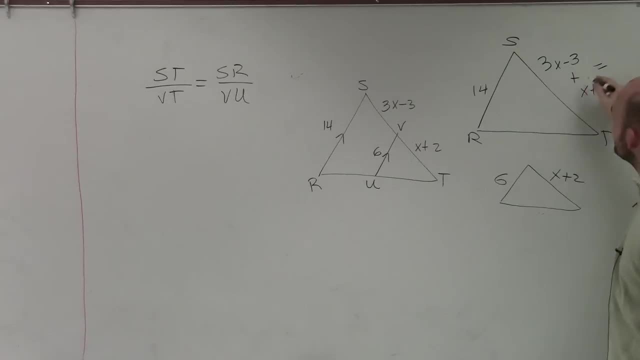 Well here this: actually, when you combine this 3x minus 3 plus x plus 2, that gives you 4x minus 1, correct? Would everybody agree with that? when I combine those, I combine the x's and combine the numbers. 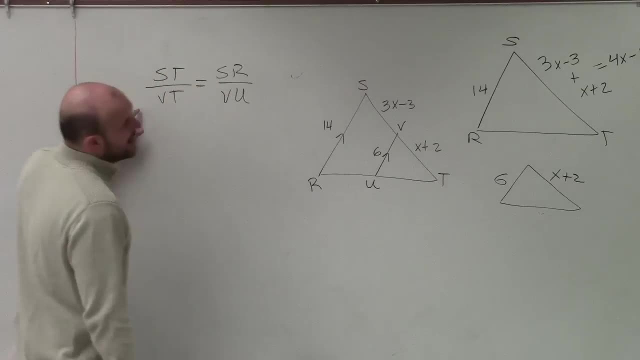 Would everybody agree with that? Okay, So I can say: ST is 4x minus 1 over VT, Which is x plus 2. Which is equal to 14 over 6.. Now that I have a proportion, do you guys feel like now we can solve this by using our cross multiplication and cross product? 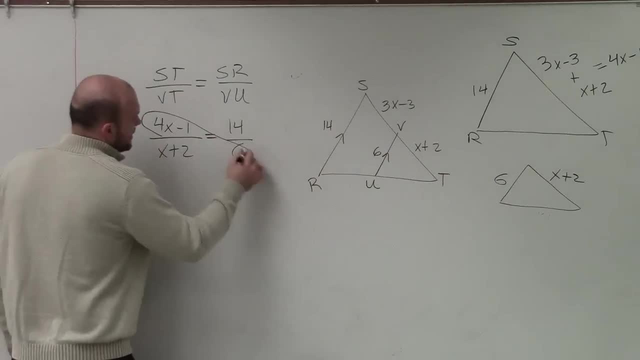 Yeah. Now it's kind of into an element where you guys are like: oh okay, I can probably do it from here now. So then I write: 6 times 4x minus 1 equals 14 times x plus 2.. 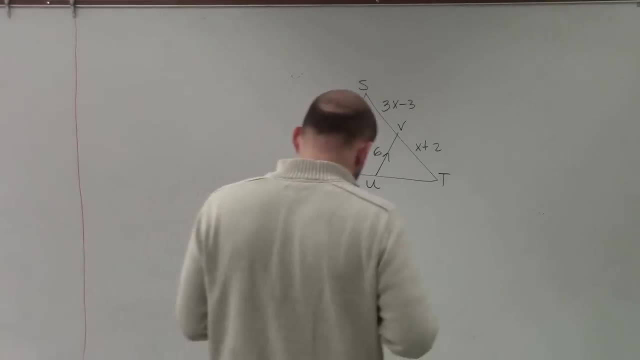 So what they're asking, ladies and gentlemen, in this problem is identify the similar triangles, then find each measure. So what we need to do again, when we're doing a problem like this, we're going to go ahead and do it. a problem like this. 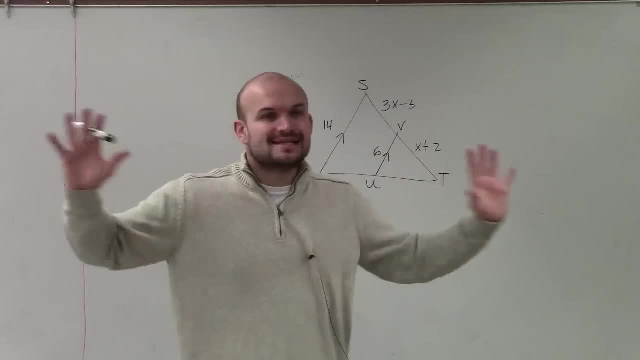 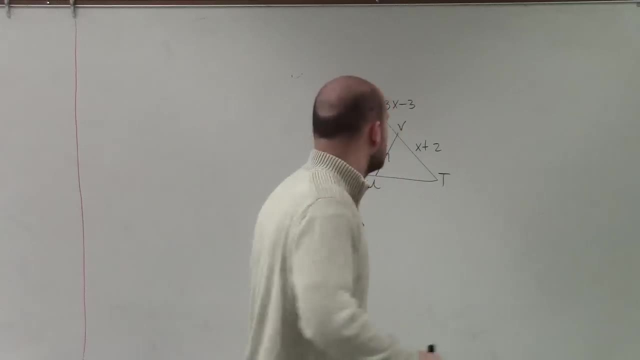 The main important thing that I told you guys is to take away the triangles right. Separate the triangles so you can see them, Carly, as their own identity, not trying to determine what is one triangle over the other. So I am going to draw them separately, all right, and then go ahead and label them SRT, all right. 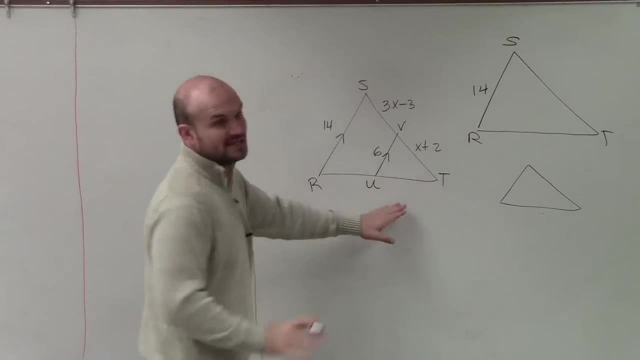 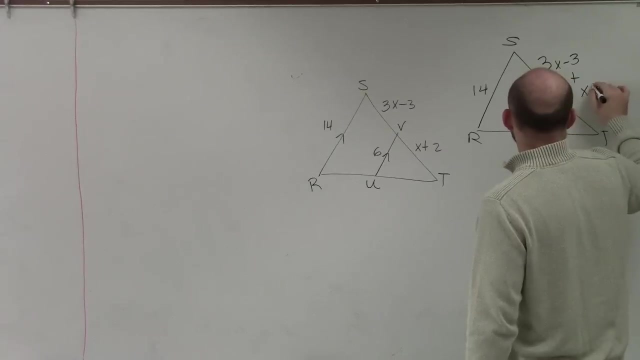 So this length is 14.. We don't know what this length is right, But we know that this length is going to be 3x minus 3 plus x plus 2.. Would you guys agree on that, Caleb, do you? 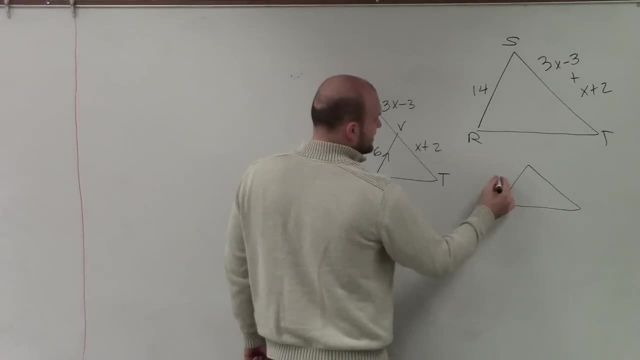 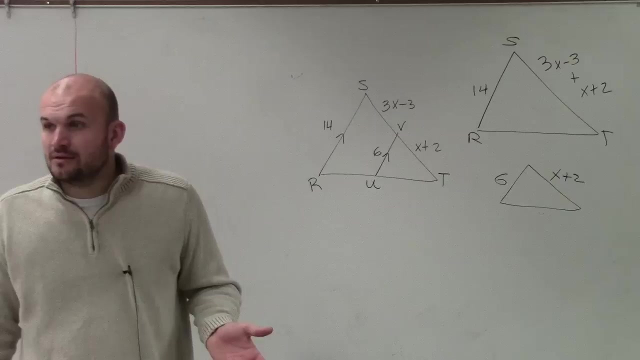 Agree on that. Okay, Over here you could say: this length is 6, and this one is x plus 2.. So what we're trying to do is they say they are similar, but how are we going to be able to? if they're similar, then that means their side lengths, right, are proportional. 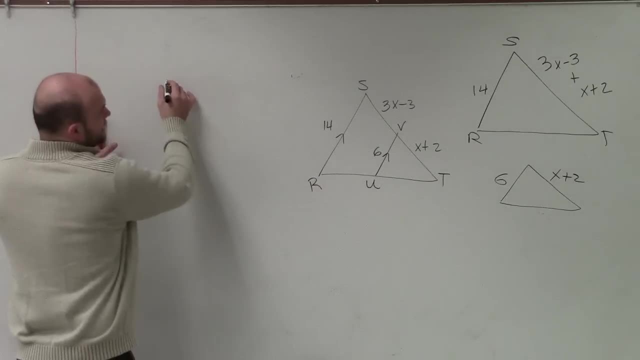 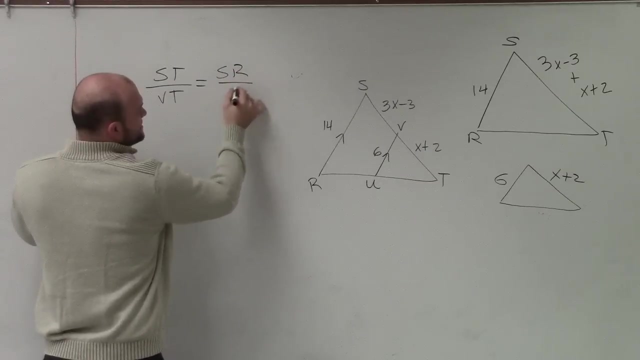 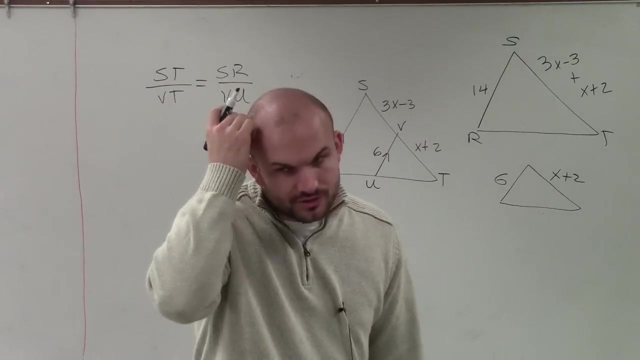 So what I can say, then is I can say: ST is to VT is equal to SR is to VU. All right, Their side lengths are going to be proportional to each other. So now what I need to do is just plug in their side lengths. 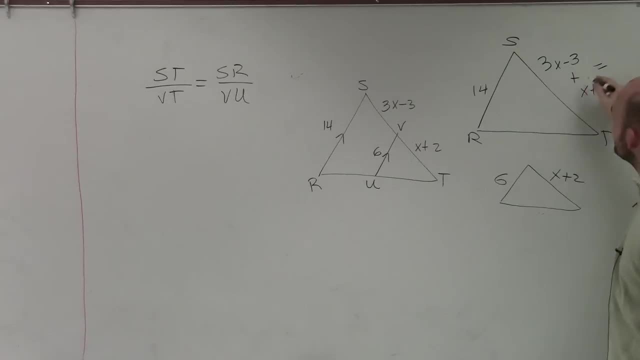 Well here this: actually, when you combine this 3x minus 3 plus x plus 2, that gives you 4x minus 1, correct? Would everybody agree with that? when I combine those, I combine the x's and combine the numbers. 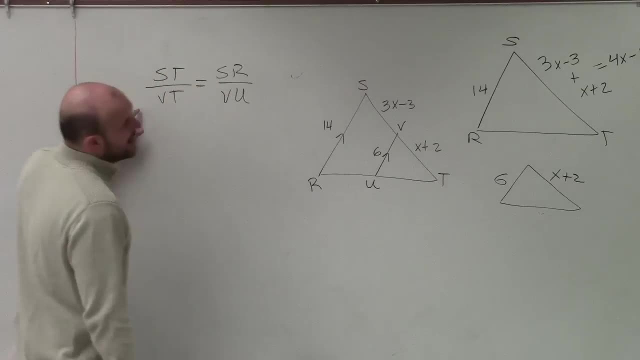 Would everybody agree with that? Okay, So I can say: ST is 4x minus 1 over VT, Which is x plus 2. Which is equal to 14 over 6.. Now that I have a proportion, do you guys feel like now we can solve this by using our cross multiplication and cross product? 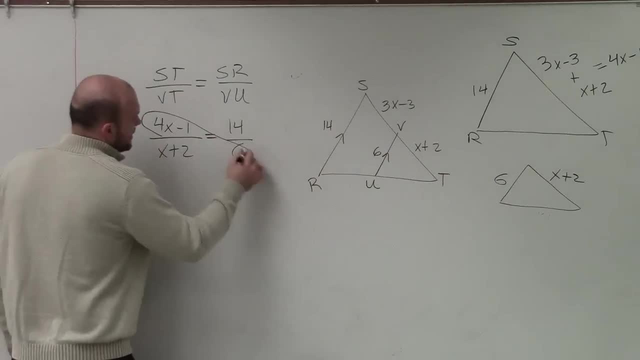 Yeah. Now it's kind of into an element where you guys are like: oh okay, I can probably do it from here now. So then I write: 6 times 4x minus 1 equals 14 times x plus 2..